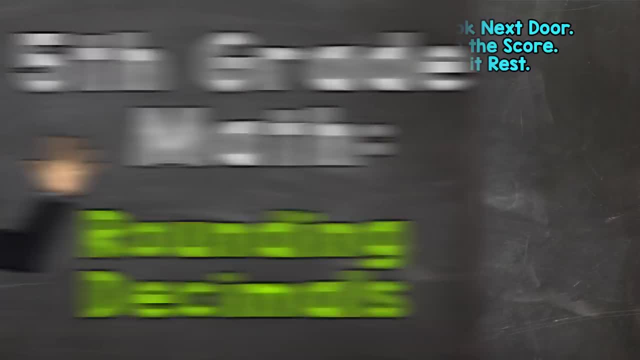 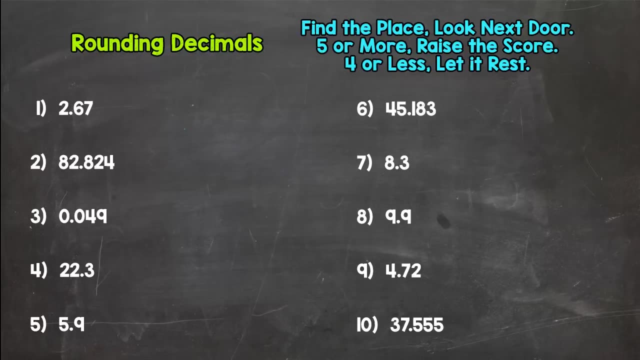 Welcome to 5th Grade Math with Mr J Alright. today we're going to be rounding decimals, And rounding decimals is very similar to rounding whole numbers. So if you know your rounding rules and how to round, this is going to be pretty easy for you. 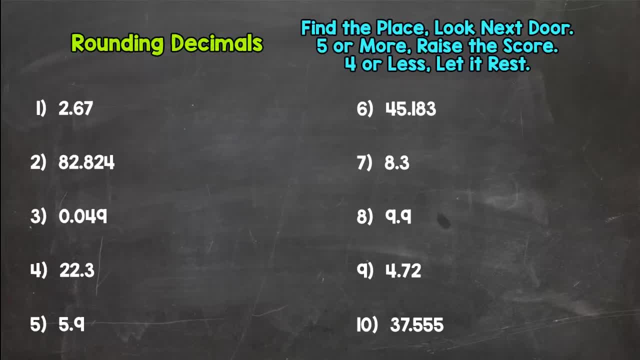 There's just a very minor difference between whole numbers and decimals, But your rounding rule is the same And if you look up to the top, right up here I put the rounding rule for a refresher So you find the place. look next door: 5 or more. raise the score 4 or less. let it rest. 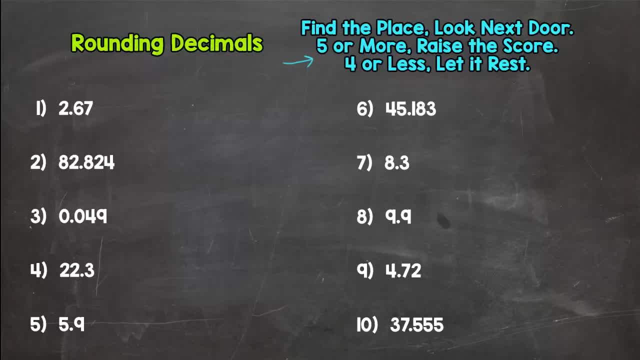 So we are going to do 10 together here for the instructional video. This is the instructional video And once we get through this 10, you can try the mastery check which I dropped the link in the description for the mastery, Where you can try 10 on your own and see if you've mastered rounding decimals. 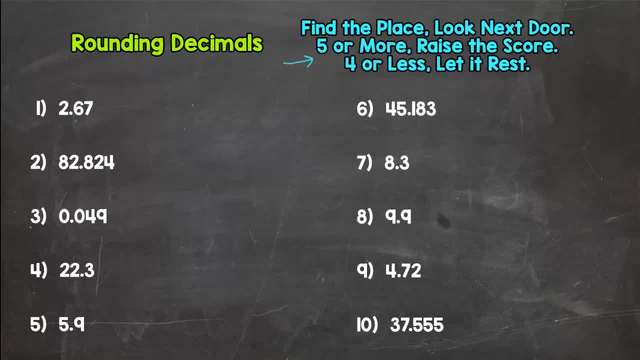 So let's hop into number 1 here And we're going to round to the underlined place. We're going to round to the tenths place for number 1.. So we have a 6th in the tenths place. We need to see if 2 and 67 hundredths rounds up to 2 and 7 tenths. 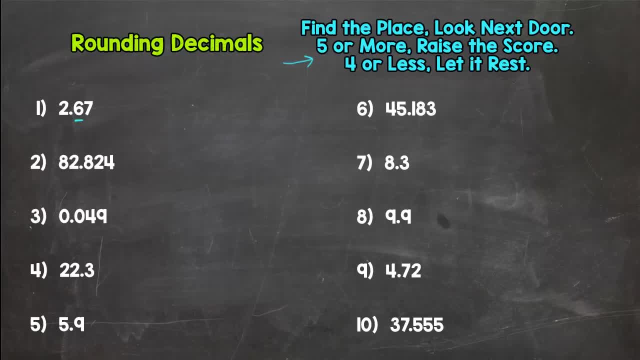 Is it closer to 2 and 7 tenths, Or is this number closer? Or is it closer to 2 and 6 tenths? Does that 6 stay the same? Well, let's look next door at this 7.. 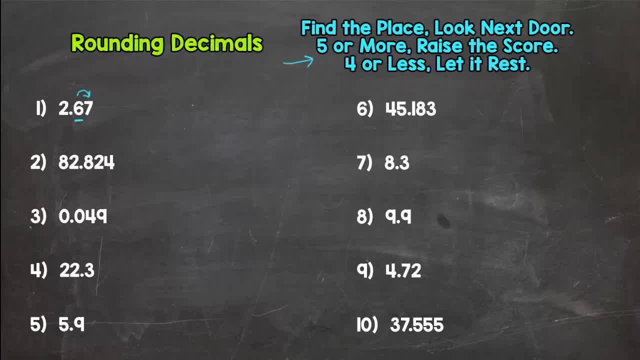 And that 7 says that this number is closer to 2 and 7 tenths. You would round up to 2 and 7 tenths. Now here's the minor difference between whole numbers and decimals. In decimals, when you round to the given place, for example, number 1 is the tenths place. 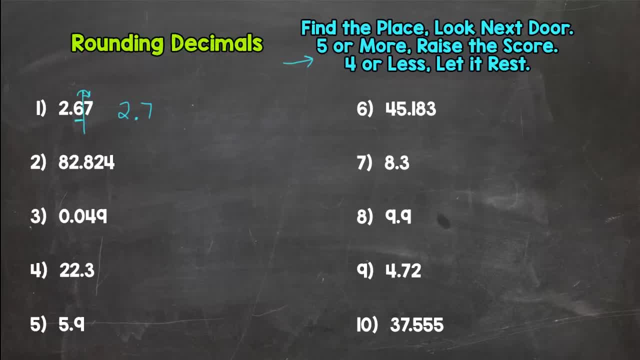 we cut it off at the tenths place. We don't fill with zeros like we do with whole numbers. So you would just put 2 and 7 tenths. You don't need to add a zero on the end. So let's do number 2.. 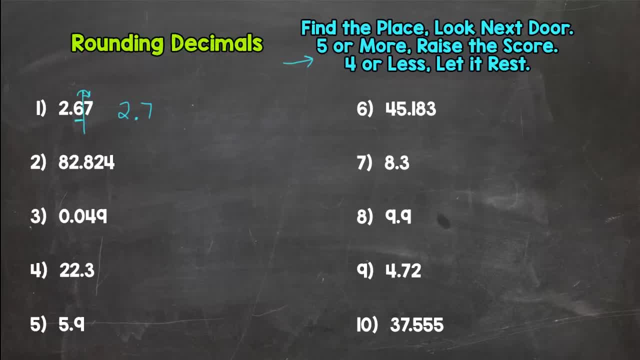 we cut it off at the tenths place. We don't fill with zeros like we do with whole numbers. So you would just put 2 and 7 tenths. You don't need to add a zero on the end. So let's do number 2.. 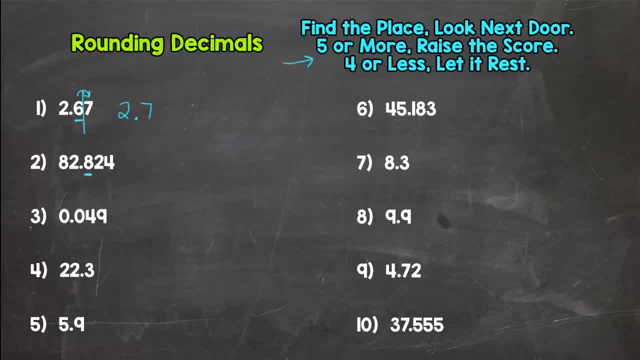 Let's do the tenths place in number 2.. So we have an 8 in the tenths place. Let's look next door. Does that 2 say round up or stay the same? Is this number closer to 2 and 8?? 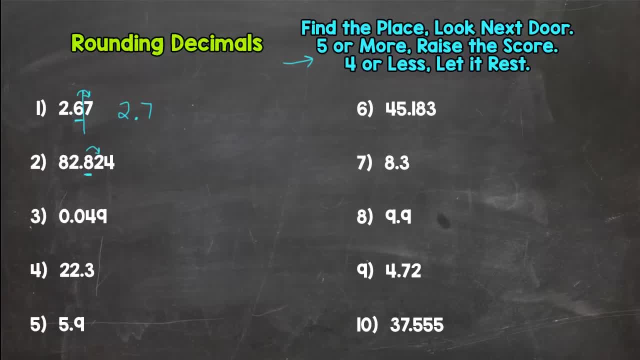 82 and 8 tenths, Or closer to 82 and 9 tenths. This 2 says: let it rest. So it will be. it will round to 82 and 8 tenths. Like I said in number 1, we cut it off at the rounded place. 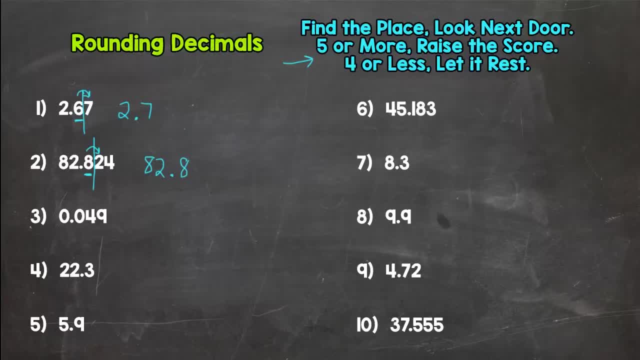 This is for decimals, only For whole numbers. you change everything to the rounded place to zeros. Here we cut it off. So let's round to the hundredths place for number 3.. So we look at the 4.. Look next door. 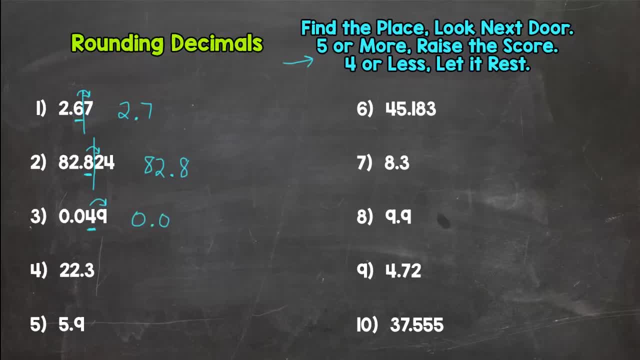 And you should be thinking to yourself: we will round up And this is closer to 5 hundredths than it is to 4 hundredths, And we cut it off at the hundredths place For number 4, let's round to the nearest whole number. 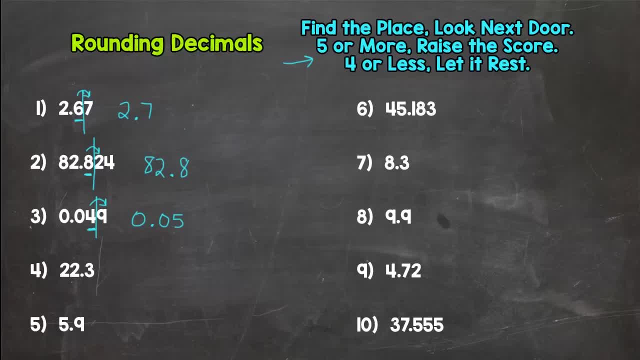 If you ever hear round to the nearest whole number, that means the ones place. So we're going to see if this number is closer to 22 or 23.. What does it round to? So let's look next door. That 3 says stay the same. 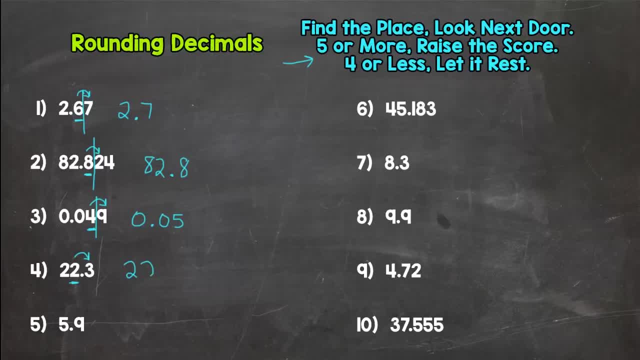 So 22 and 3 tenths rounds to 22 for the nearest whole number. Let's do nearest whole number for number 5 as well. So we have a 5 and 9 tenths here, And when I say, let's round 5 and 9 tenths to the nearest whole number. 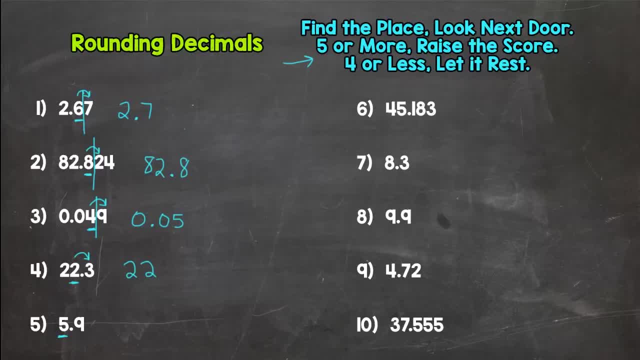 it's basically asking: is this number closer to 6 or 7, or, I'm sorry, 5 or 6.. So let's look next door And that 9 says: add one more or round up, So we would round to 6.. 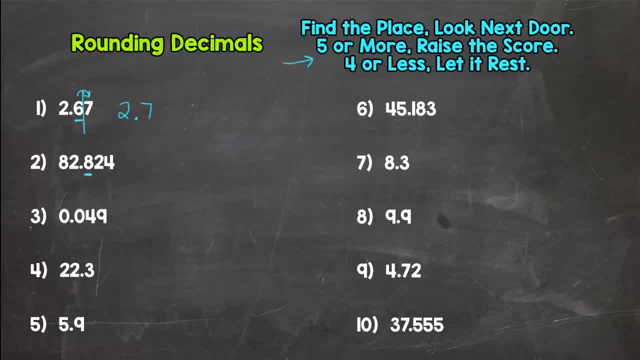 Let's do the tenths place in number 2.. So we have an 8 in the tenths place. Let's look next door. Does that 2 say round up or stay the same? Is this number closer to 2 and 8?? 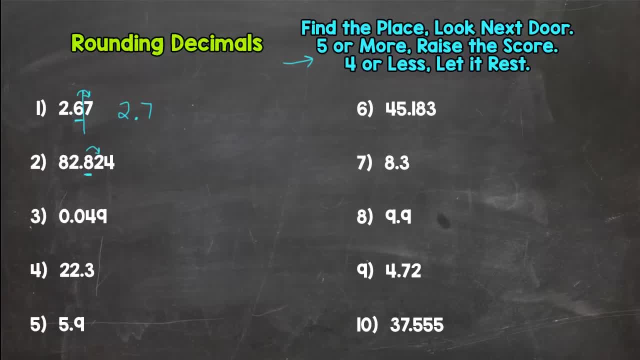 82 and 8 tenths, Or closer to 82 and 9 tenths. This 2 says: let it rest. So it will be. it will round to 82 and 8 tenths. Like I said in number 1, we cut it off at the rounded place. 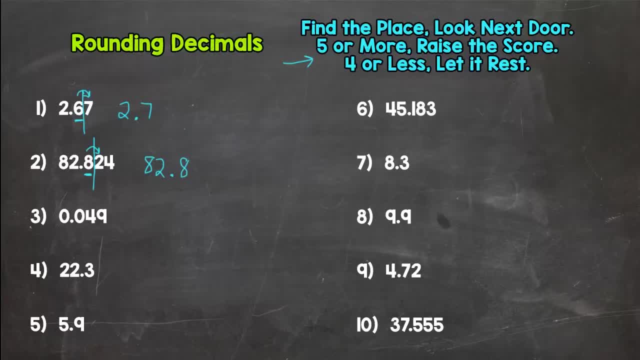 This is for decimals, only For whole numbers. you change everything to the rounded place to zeros. Here we cut it off. So let's round to the hundredths place for number 3.. So we look at the 4.. Look next door. 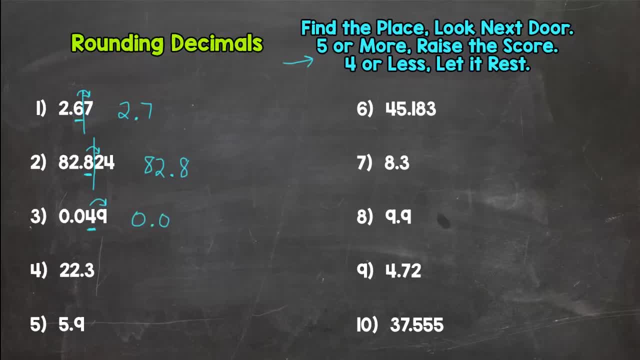 And you should be thinking to yourself: we will round up And this is closer to 5 hundredths than it is to 4 hundredths, And we cut it off at the hundredths place For number 4, let's round to the nearest whole number. 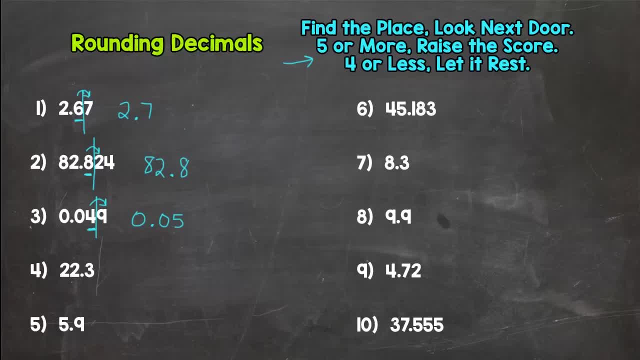 If you ever hear round to the nearest whole number, that means the ones place. So we're going to see if this number is closer to 22 or 23.. What does it round to? So let's look next door. That 3 says stay the same. 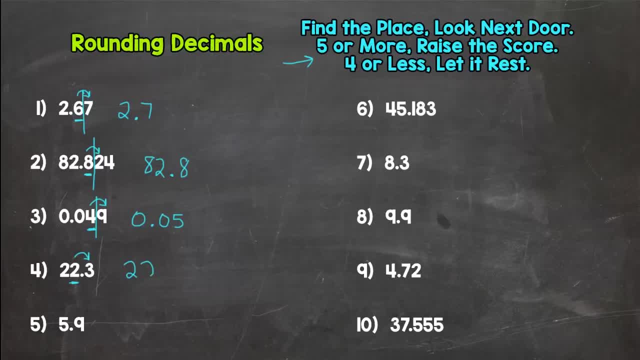 So 22 and 3 tenths rounds to 22 for the nearest whole number. Let's do nearest whole number for number 5 as well. So we have a 5 and 9 tenths here, And when I say, let's round 5 and 9 tenths to the nearest whole number. 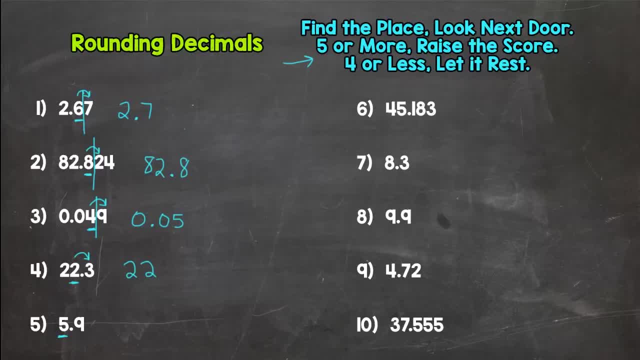 it's basically asking: is this number closer to 6 or 7, or, I'm sorry, 5 or 6.. So let's look next door And that 9 says: add one more or round up, So we would round to 6.. 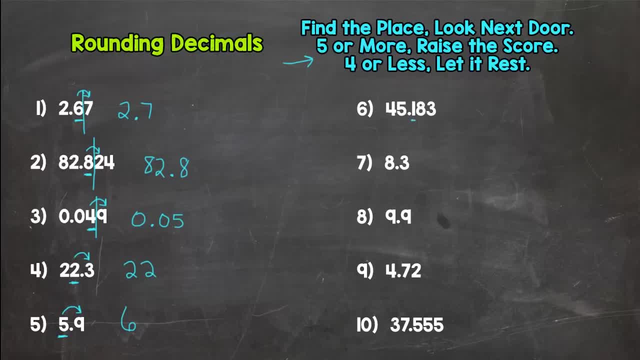 Alright, let's go to number 6.. Let's round to the tenths place again. So we have a 1 in the tenths. Let's look next door And we have an 8. So that says round up. So we should have 45 and 2 tenths. 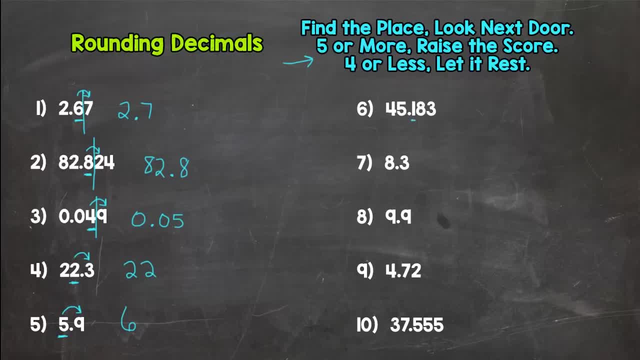 Alright, let's go to number 6.. Let's round to the tenths place again. So we have a 1 in the tenths. Let's look next door And we have an 8. So that says round up. So we should have 45 and 2 tenths. 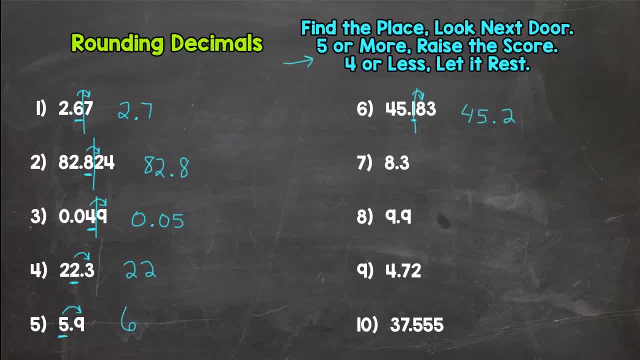 And remember: cut off at whatever decimal place they tell you to round to. For number 7, let's do nearest whole number. So is this 8 and 3 tenths closer to 8 or 9?? Next door, That 3 says stay the same. 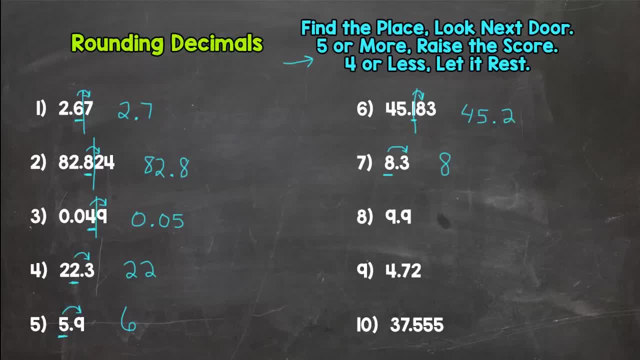 So that number would round to 8.. 8 would be the nearest whole number. Let's do nearest whole number again for number 8 here. Look next door. So are we going to round up to 10? Or is 9 and 9 tenths closer to 9?? 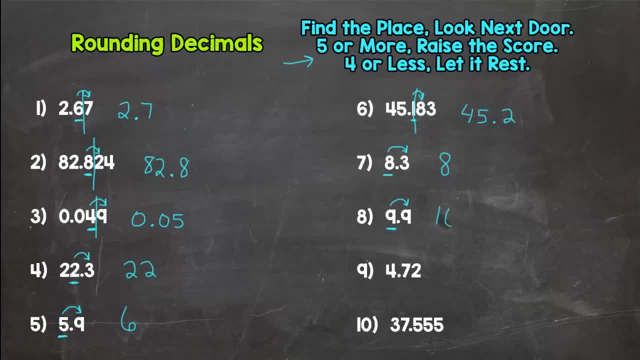 Well, 9 says round up, So this number 9 and 9 tenths would round to 10. if you are rounding to the nearest whole number, Number 9,, let's round to the tenths. Let's look next door. 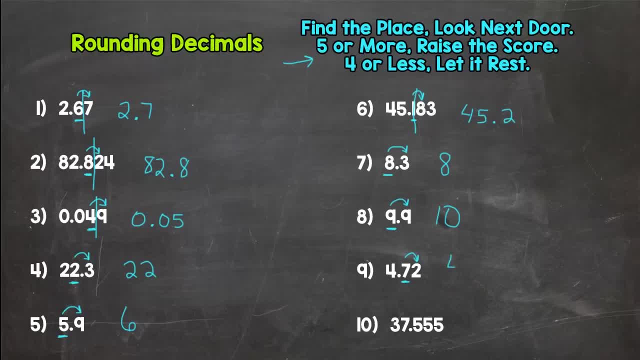 2 says: stay the same. So you would round to 4 and 7 tenths if you were to round to the nearest tenths And then number 10, let's do the hundredths place. Okay, look next door. 5 says add one more or raise the score. 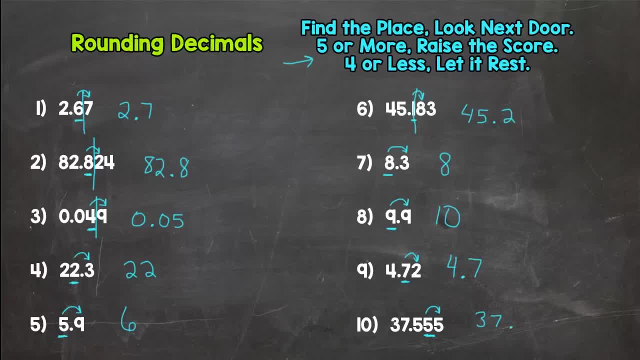 So we have 37 wholes and 56 hundredths. if you were to round to the hundredths And remember, cut off at the rounded place. So maybe you're just learning about rounding decimals, Or you needed a refresher, Or you're studying for a test. 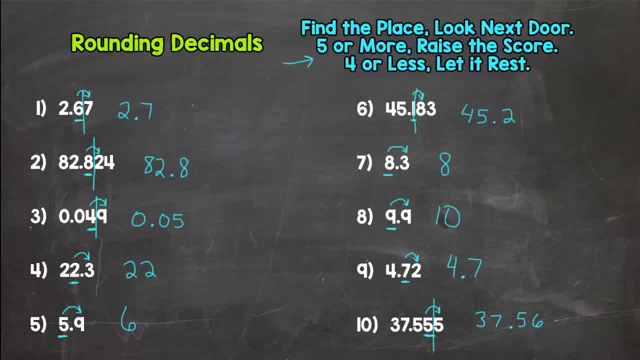 Whatever it is, hopefully that helped out with rounding decimals. My advice would be checking out the mastery check video next, Which, like I said, is in the description, So click on that link. You're going to try some on your own. 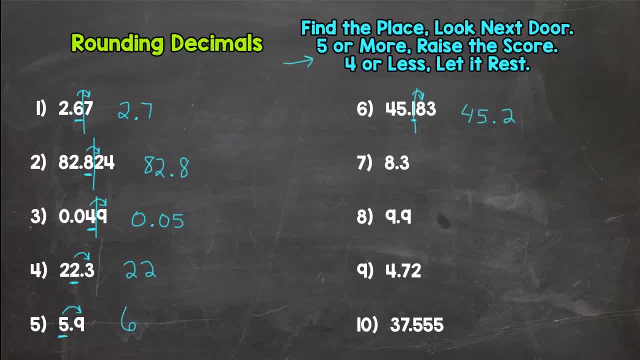 And remember: cut off at whatever decimal place they tell you to round to. For number 7, let's do nearest whole number. So is this 8 and 3 tenths closer to 8 or 9?? Next door, That 3 says stay the same. 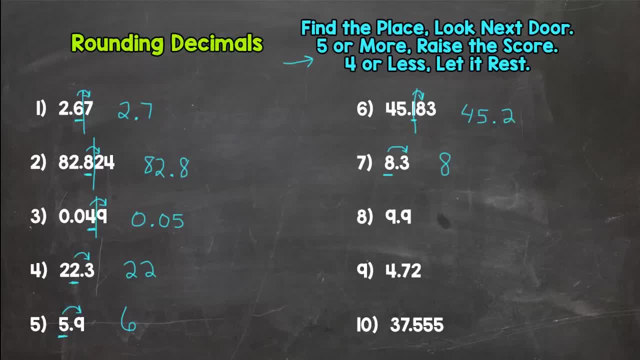 So that number would round to 8.. 8 would be the nearest whole number. Let's do nearest whole number again for number 8 here. Look next door. So are we going to round up to 10? Or is 9 and 9 tenths closer to 9?? 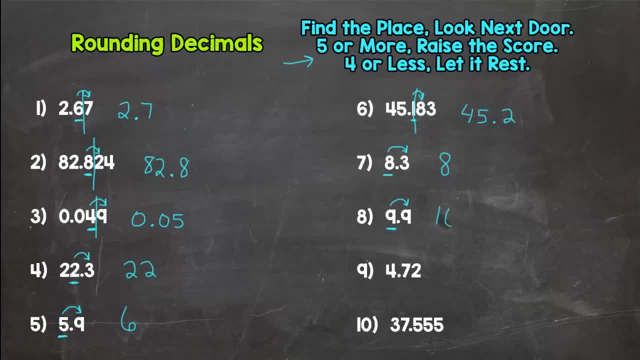 Well, 9 says round up, So this number 9 and 9 tenths would round to 10. if you are rounding to the nearest whole number, Number 9,, let's round to the tenths. Let's look next door. 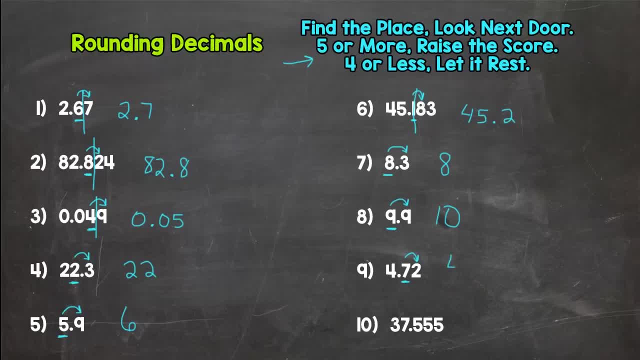 2 says: stay the same. So you would round to 4 and 7 tenths if you were to round to the nearest tenths And then number 10, let's do the hundredths place. Okay, look next door. 5 says add one more or raise the score. 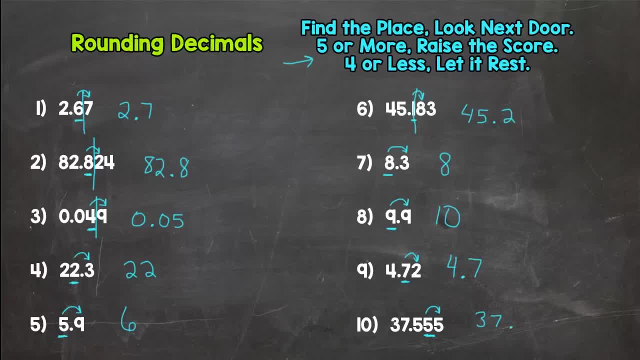 So we have 37 wholes and 56 hundredths. if you were to round to the hundredths And remember, cut off at the rounded place. So maybe you're just learning about rounding decimals, Or you needed a refresher, Or you're studying for a test. 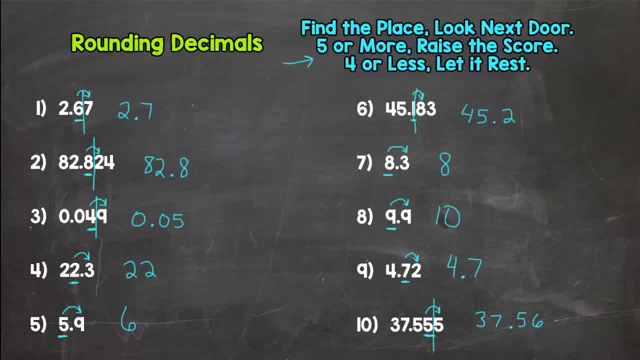 Whatever it is, hopefully that helped out with rounding decimals. My advice would be checking out the mastery check video next, Which, like I said, is in the description, So click on that link. You're going to try some on your own. 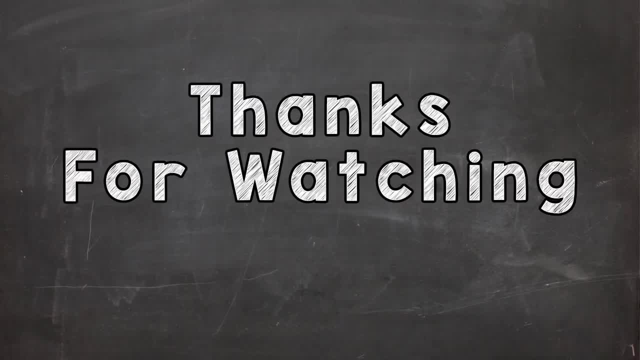 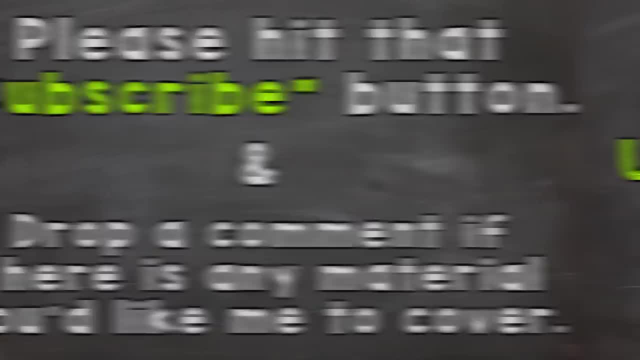 And see if you have it down. Thanks for watching. Please hit that subscribe button And drop a comment if there's any material you'd like me to cover. Until next time, peace.